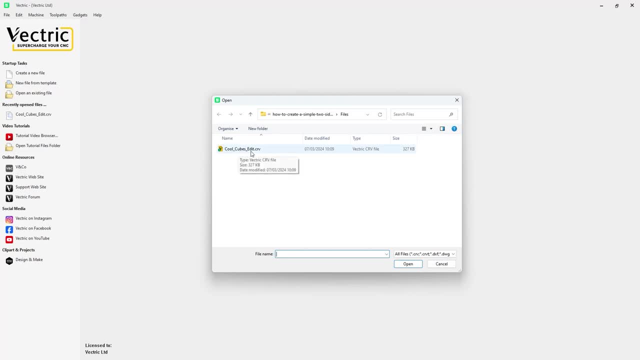 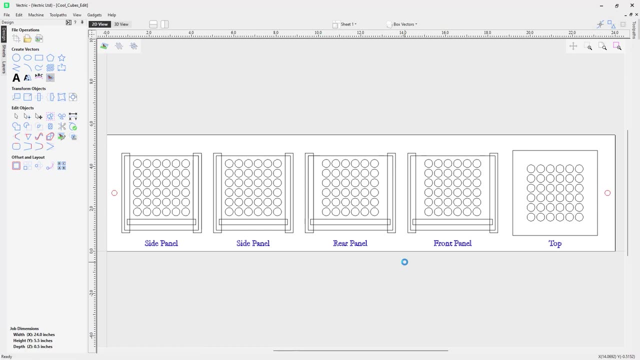 you'll see a file called cool underscore cubes- underscore edit, dot crv. So we'll select that and we'll open this up Now, right away you're going to see we have five different sides of our cool cube. The bottom panel is missing because it's a really basic square. 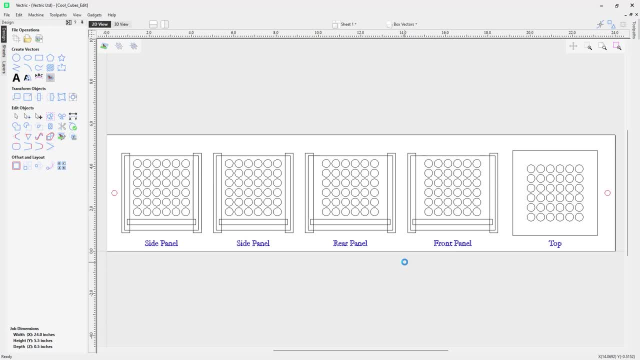 that we assume that you'll be able to create on your own. You'll see, we have a side panel, another side panel, a rear panel, a front panel and then a top panel. We also have two holes here that represent dowel holes, and we'll talk about those in a bit. On the 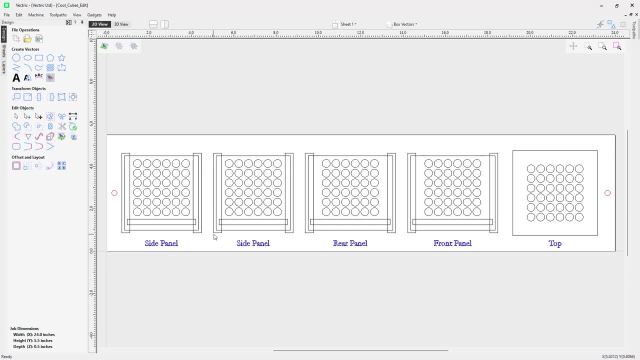 top side of our project we'll be cutting the slots to accept the side panel so we can glue it all up, And on the bottom side we'll actually be cutting these decorative circles and also we'll be using it to cut out these panels. So the outside square will be our. 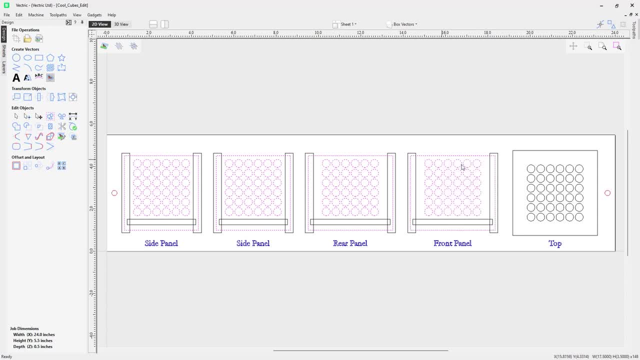 cutout profile toolpath to cut out the panels so we can assemble this box together. Now, as this file starts out, it's only a side panel, so we're going to cut out the bottom side panel, and then we're going to cut out the top side panel, and then we're going to 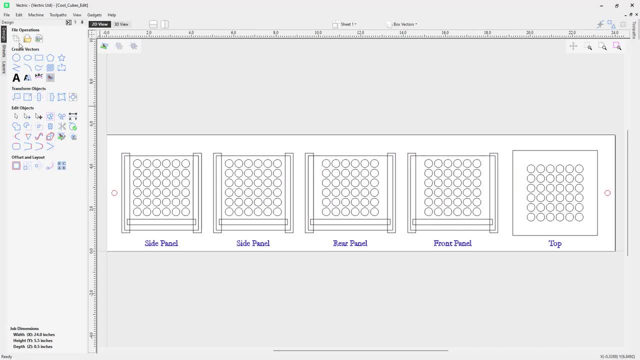 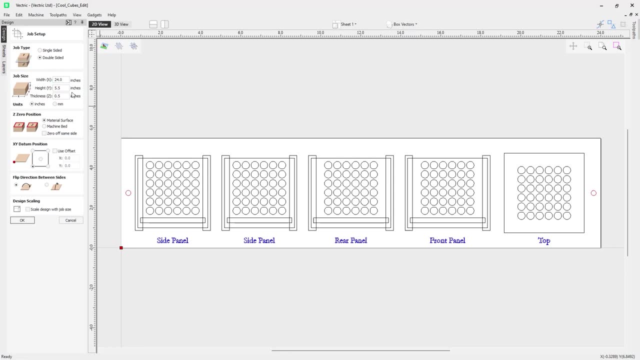 do the same thing. So we're going to go into our toolpath and we're going to change this to a single sided job. So our first step is to go into our job setup and change it to a double sided job. Now, everything here is going to stay exactly the same in our job. 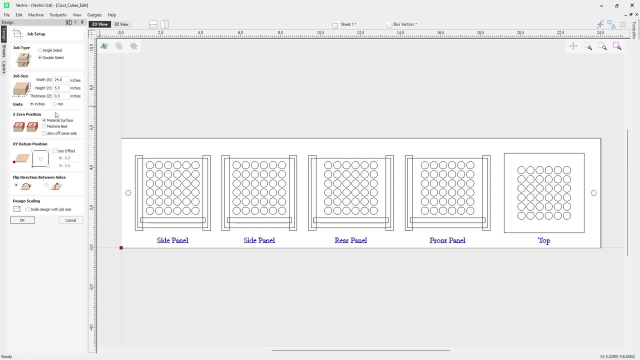 size as it was in the original file. But we're going to change where we're going to be zeroing our tool off of our material. We're going to be zeroing off the same sides, So we're going to be zeroing off our material surface on the top side And that's so we can reference. 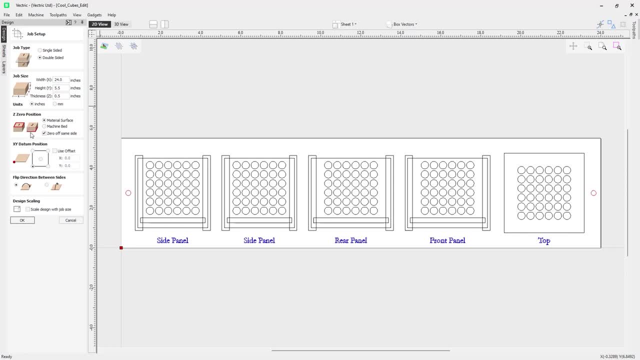 the same side of that material. We're going to be zeroing off our machine bed. for the second side, Which is actually the top side of our material, The data must be staying the same. We're going to be flipping left to right, but we do have the option to flip from bottom to top, Just. 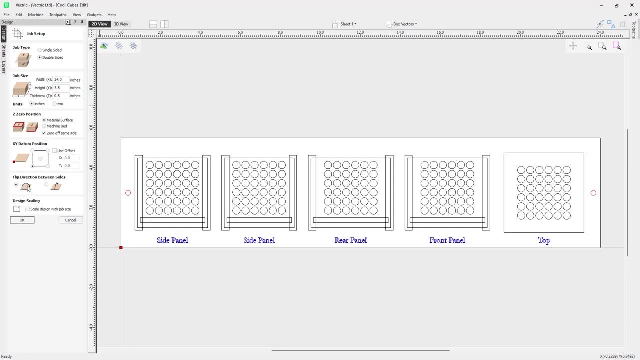 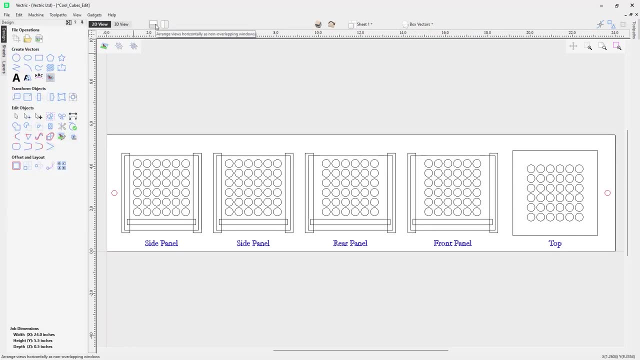 remember the way this area was facing right now, because we'll look at that in a second later on in our interface And we can just go ahead and click OK Now we'll go ahead and tile our views. That'll make things a little bit easier for us to see So in our 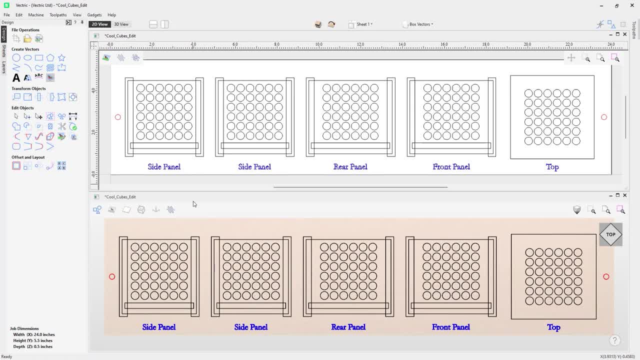 top panel we have our 2D view And in our bottom panel we have our 3D view. You'll notice we have some new icons that have shown up. This first icon will toggle on and off our double-sided view, Not only in our 2D view and our 3D view, but also when. 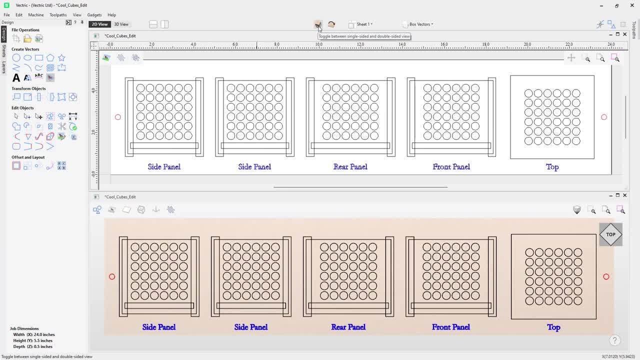 it comes to previewing our tool paths in full 3D with the front and back in situ. This icon here shows us the direction of flip. It's left to right, Just like we had set up in our job setup. If we need to change it to bottom, to top, we can go back into our job. 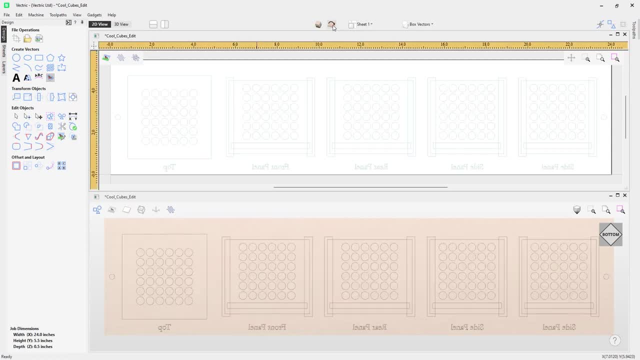 setup And just go ahead and click OK. Now we're going to go ahead and click OK, Now we're going to just flip that around. You'll notice that when we flip to our backside of our job in our 2D view, we can tell right away that we're in our backside of our project because the 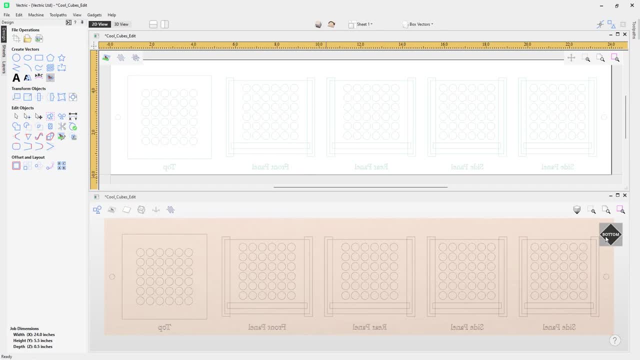 rules are now a different color And in our 3D view you'll notice that our view control now has a black bold square around the text bottom, And so if I go ahead and just double click on that, it'll flip us to the top And you see, the top doesn't have that black border. 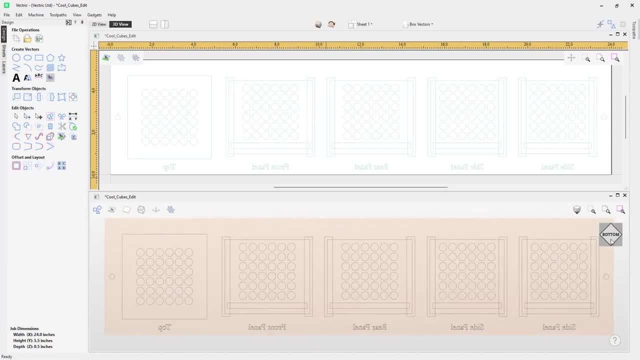 So we can just go ahead and flip back to the other side again. I'm sure you've already noticed that I can see the vectors from the top side of my job on the bottom side. This is really handy when it comes to referencing where my vectors are. 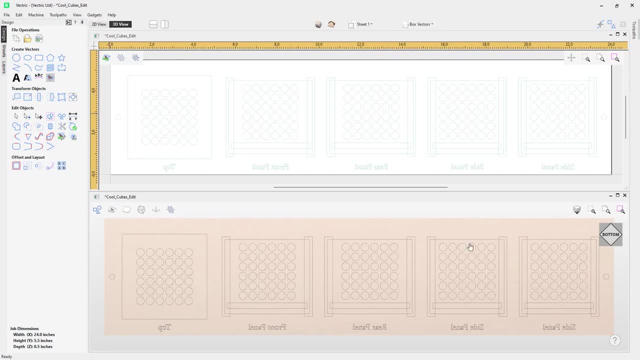 on the other side of my material And, as you can see here, they are a light gray or a light green And I can't actually select them from the opposite side of my job. I need to be on the side of the job that those vectors are on. 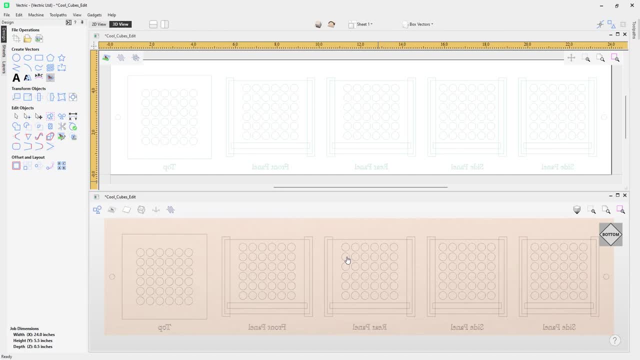 This is also a good time to point out that our snapping will reference geometrically on the other side of our job if we have our double-sided view turned on. So from here, most of our work can be done with just a 3D view. So let's just go ahead. 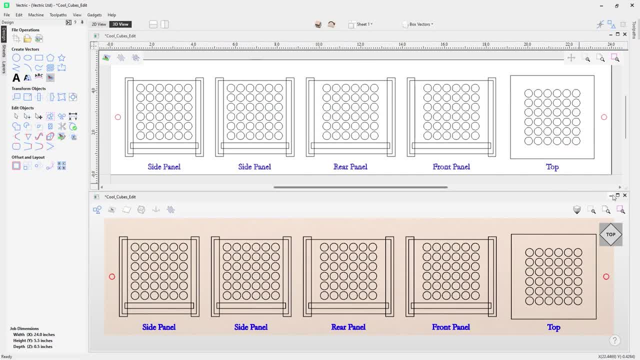 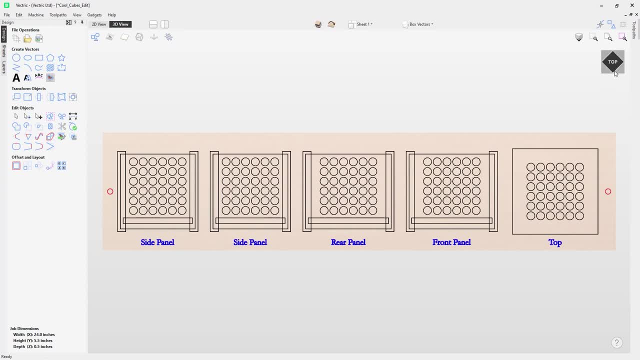 and flip over to our top side of our job again and maximize our 3D view. I want to point out again that, because this is a double-sided job, that the top indicator on our view control has been outlined in black, So we know that we're on the top side of our 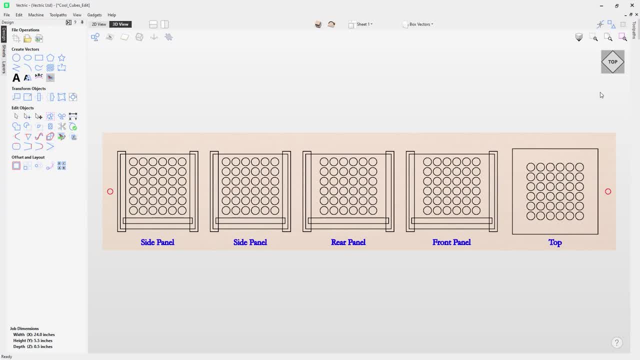 job in our 3D view. Our next step is going to be to organize our file a little bit. So we're going to want to select and move all of our vectors that we want to cut on the bottom of our material to the bottom side of our job. So to do that, I'm going to go ahead and marquee select. 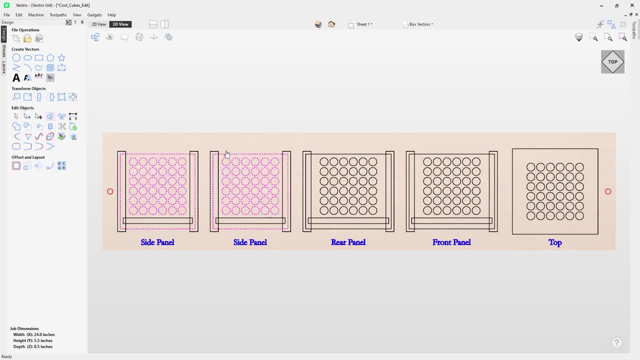 holding down my shift key. all the decorative circles and the outside square that we're going to be using as our profile cut to cut out our panels, And then we'll right click on those, Go down to move to other side, And you see, as soon as I do, that they become that gray. 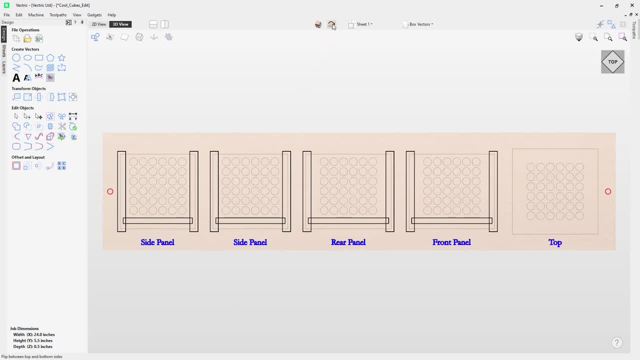 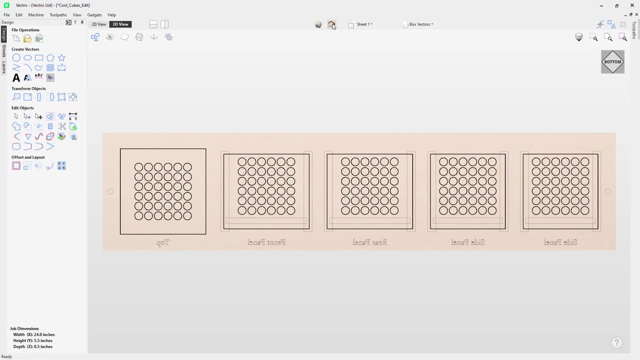 color because they're on the other side of our job. If we go ahead and flip to our other side of our job, you'll see that there they are And the vectors on our top side have now been grayed out. I can also go ahead and turn off my double-sided view so that I can hide those vectors on the. 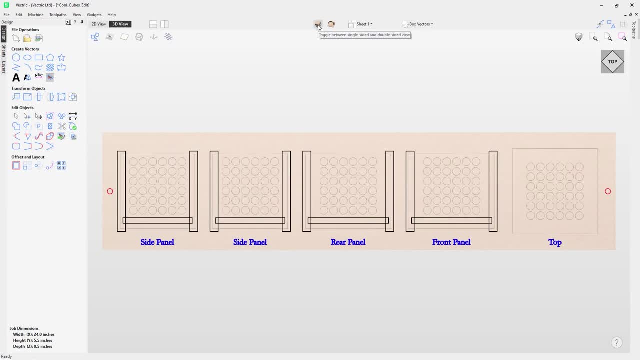 bottom side. Let's turn those back on for now. Now we have everything that we need to go ahead and move to the other side of our job. We need to go ahead and to start some tooling. So let's do that. Let's go over to our tool. 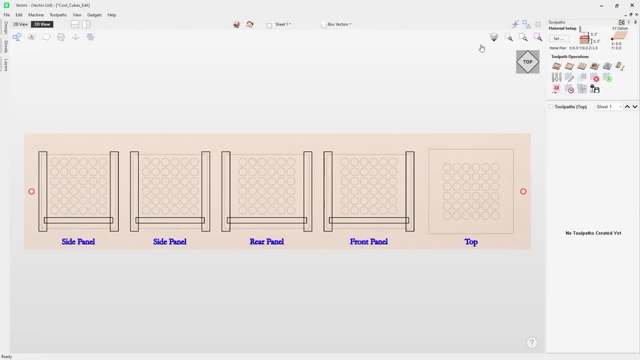 paths tab. So the first thing we're going to do, as always, is to check out our material setup. So the thickness of material is a half inch, Our datum is going to be set to the bottom left hand corner And, because we're cutting the top side of our job, we're going to be zeroing. 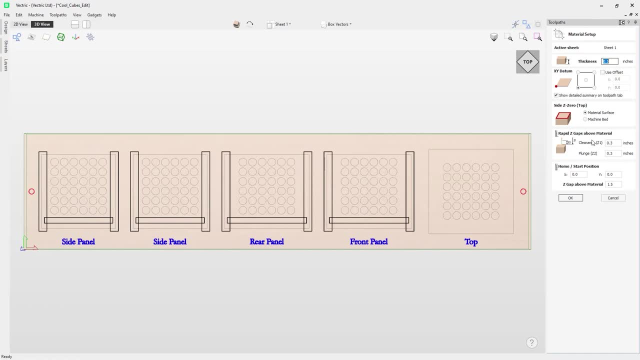 off our material surface. Our rapid Z gaps above our material and our home start position are safe and appropriate for our machine and the material we're using. So we're just going to go ahead and click OK First off. we'll go ahead and choose these horizontal pockets And we'll create a pocket. 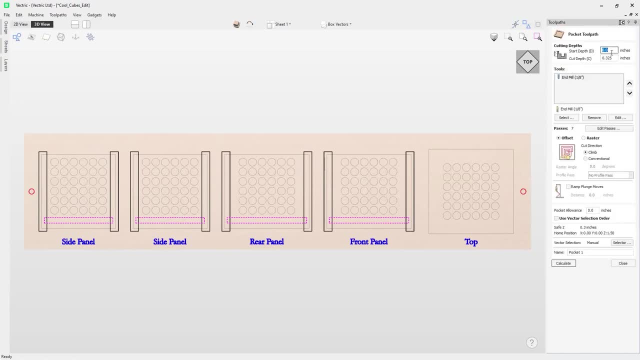 tool path. Our start depth is going to be zero. We're going to cut down an eighth of an inch. We're going to be using a quarter inch end mill, So we're going to remove this bit out of there and we'll select a brand new one out of our tool database. Make sure. 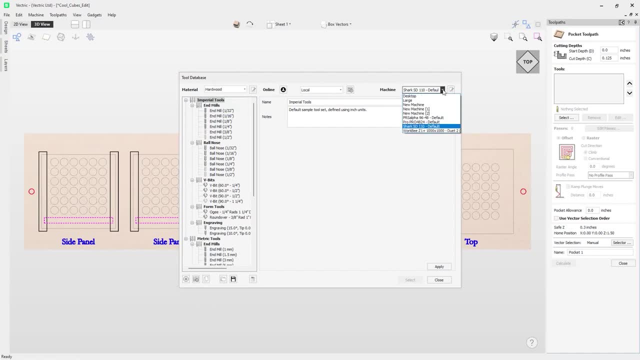 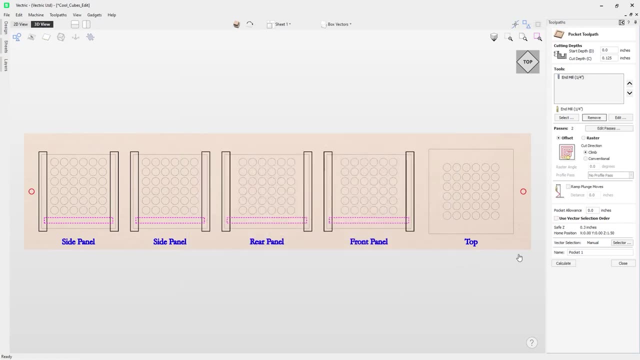 that we choose the right material, Make sure that we choose the proper machine, And we'll go ahead and grab that quarter inch end mill and select that. OK, We're going to use a raster tool path And we're going to raster back and forth. 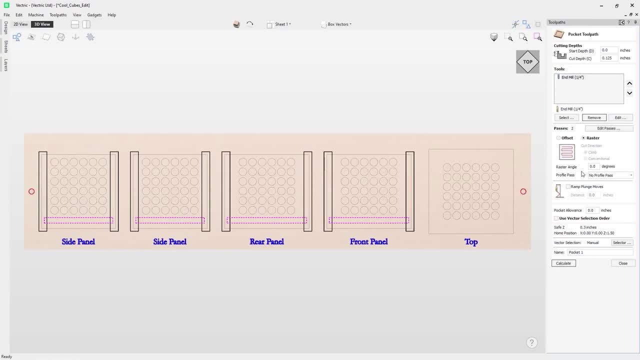 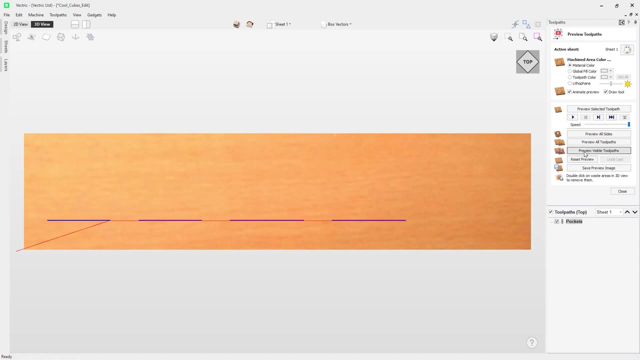 So we're going to leave our raster angle at zero And we'll set our profile path to last And we'll just rename this pockets, We'll calculate that, OK, And then we can preview that visible tool path. You see, there, we have it right there. 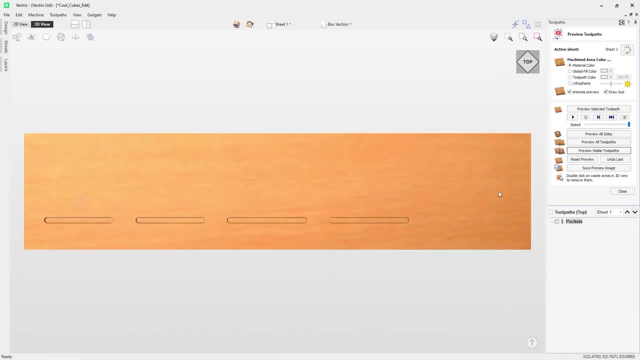 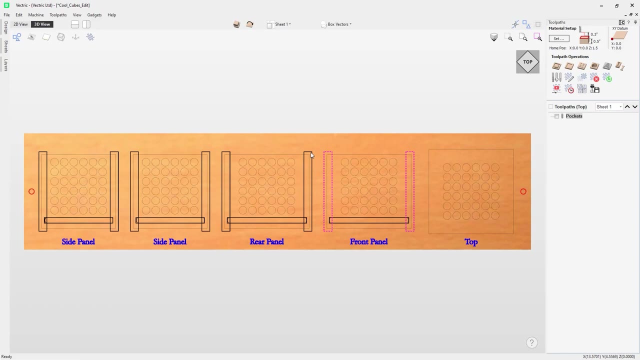 That's great. Let's look back down on the top of that again. Let's close that down. Let's go ahead and select these upper. Let's just go ahead and select the vertical pockets that we need to assemble our box. We'll choose the pocket. 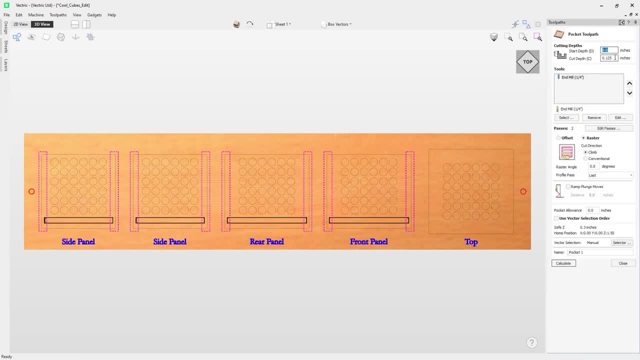 tool path again. This time we're going to cut a little bit deeper. We're going to cut down a quarter inch. Use that same end mill. This time around, though, we're going to change our raster angle to be 90 degrees. That way they'll cut up and down, And we just go ahead and we'll call. 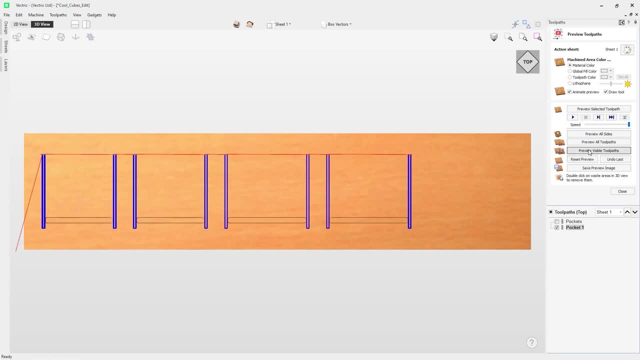 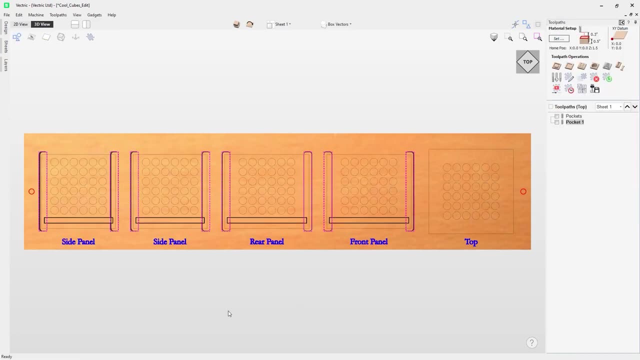 that pocket one And we'll calculate that And we can preview that visible tool path. Let's close that down Now. the last thing we're going to need to do is to create our dowel holes. So we'll select these two circles by holding down our Shift key and we're going to use our drill. 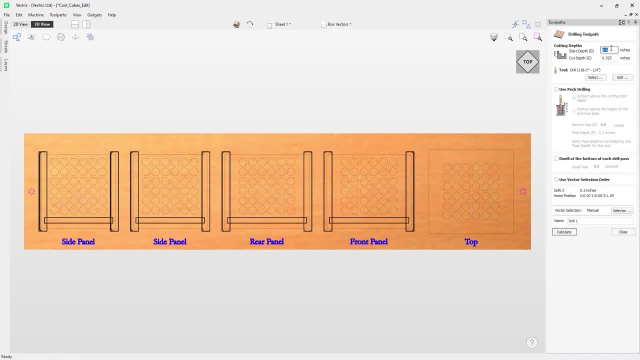 tool path for this. We're going to have a start depth of 0 and in this case we want to cut all the way through our material and straight into our spoil board. So we're going to go ahead and cut down one inch. We'll use this drill bit, It'll be fine And we'll go. 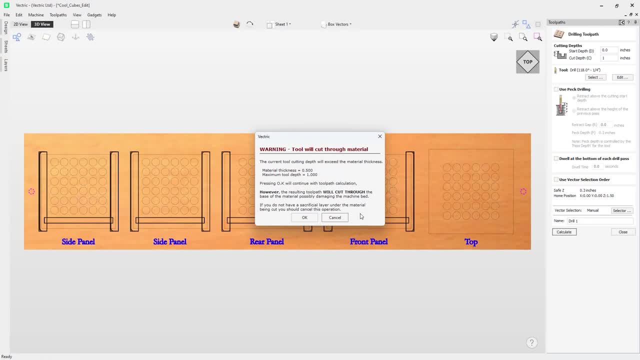 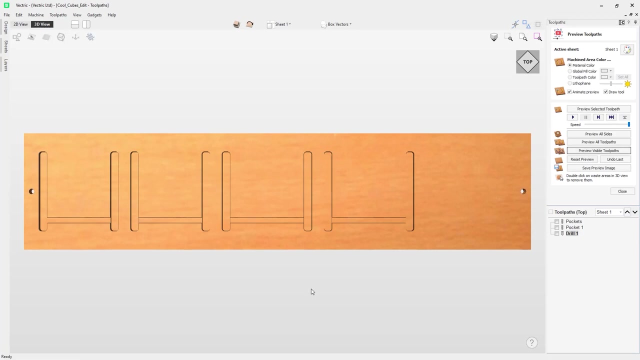 ahead and select calculate, We'll be thrown up this warning And we already know that cutting through our material into our spoil board. so that's okay. so I'll select okay, then we can preview that visible tool path. so when we get around to cutting these tool paths on our machine, we're gonna cut these three tool. 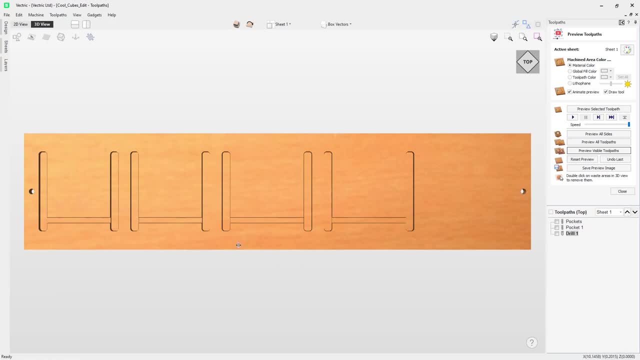 paths, and then we're going to take our material off our table and we're gonna insert in our dowels into the holes that are now into our spoil board. we'll flip our material left to right like we had set up in our job. set up and, if you 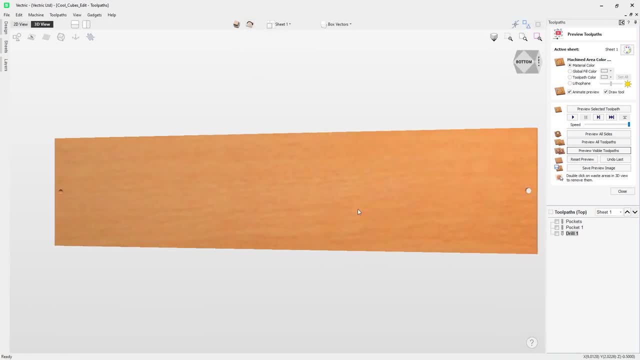 forget that, then obviously we can look at this icon right here, put that material back down on our machine and then continue to cut the tool paths that we're going to create on the backside of our job. let's go back to the top of our material. there we have it. that looks great. let's look back down on our top. 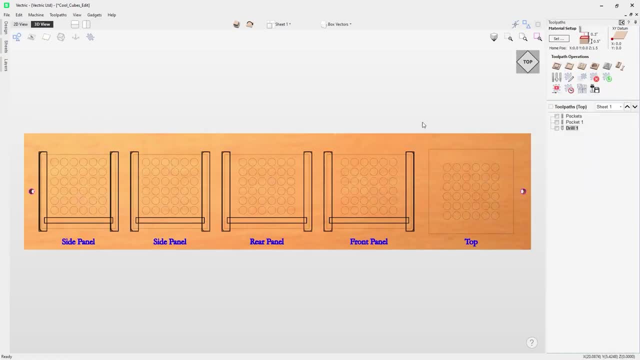 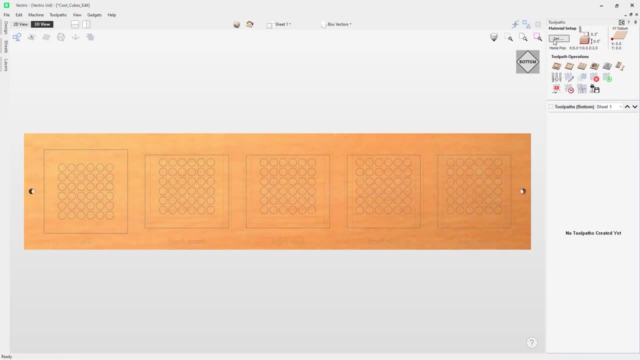 again. let's close down our tool path preview and let's flip over to our bottom side of our material. okay, now that we've finished cutting our material, let's go back to our tool path preview and let's flip our job over. let's go ahead and check our material setup again. 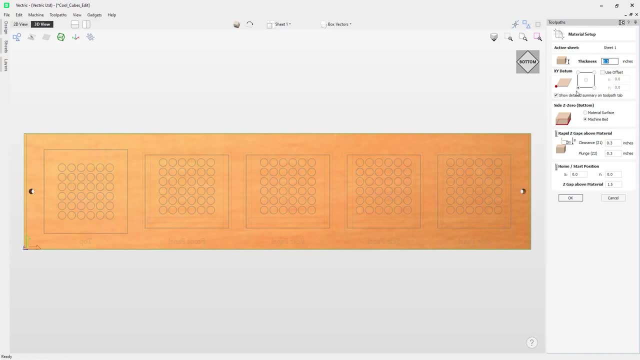 okay, our thickness of material is still at a half an inch datum, set to the bottom left corner, like it should be, but you'll see that we are now going to be zeroing off our machine bed. remember when we set up our job we said we'd 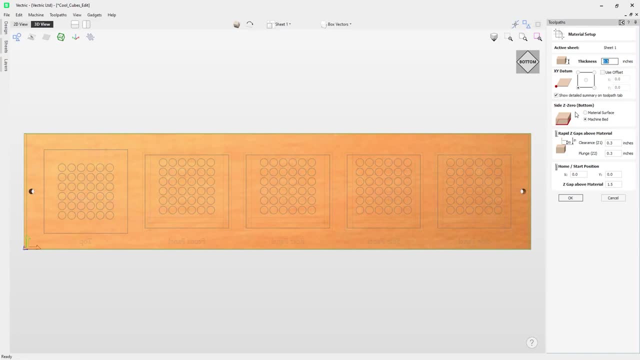 always be setting our Z zero off the same side of our material. so in this case, when we flip our material over, the face of our material is against our machine bed. also, you'll notice that in our pictorial here that the red vector is at the bottom of our material and notice that. 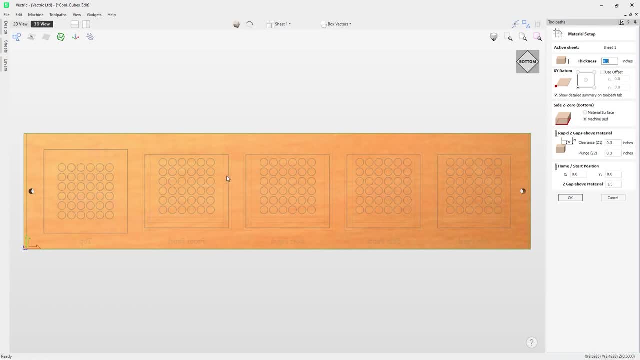 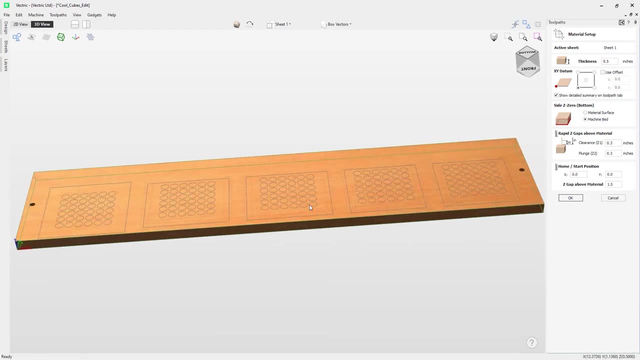 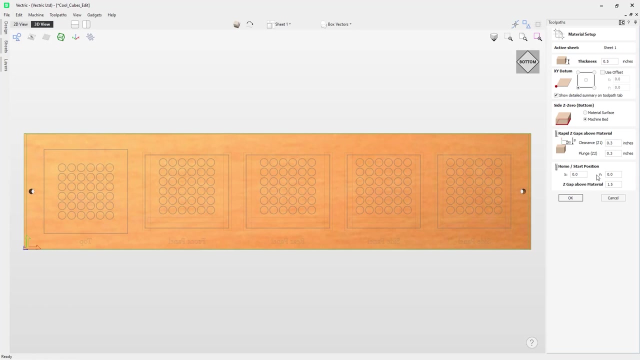 in our 3D view our vectors are slightly lighter than they were on the other side. again, this shows off that we are zeroing off our machine bed, not the top of our material. our rapid Z gaps and our home start position are safe and appropriate for the side of our material, so we can just go ahead now and click OK. 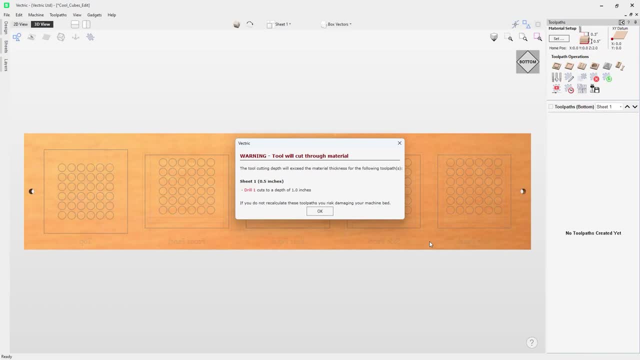 again, we'll be warned that those drill holes are going to be cutting all the way through our material and more, and we know that. so that's okay. let's just go ahead now and choose all of our circles. so, holding down our shift key, we're just going to marquee, select all of our 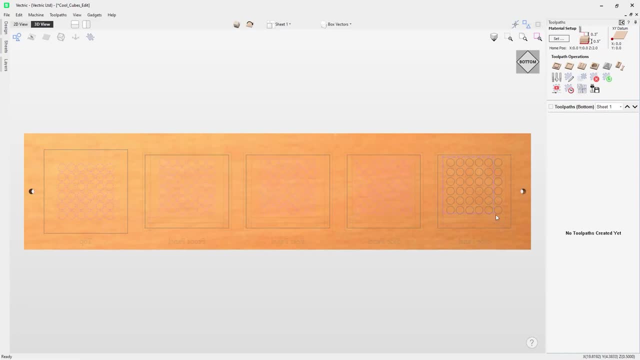 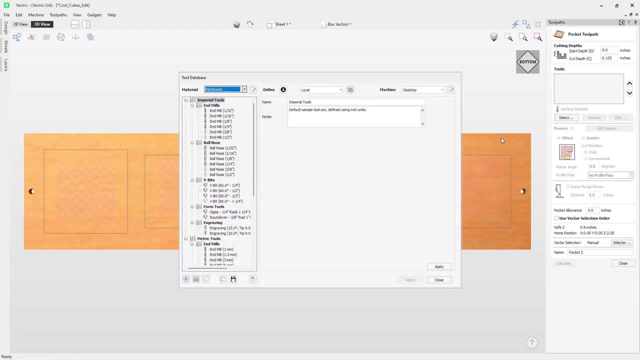 circles. then we're going to choose our pocket tool path. we start at zero and we're going to cut down an eighth of an inch. we're not going to use an end mill, so we'll remove that and we'll select a brand new tool. we're going to use a quarter inch ball nose, so we'll select that. 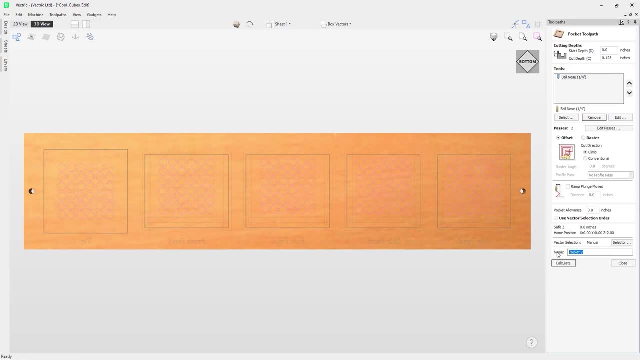 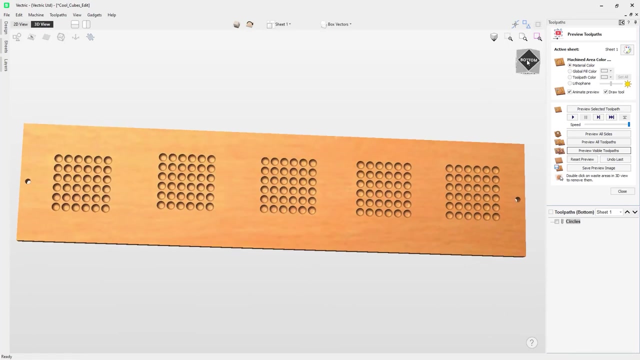 we use offset tooling and we're going to go and call this circles and we'll calculate that, and more previewer, visible tool paths and those look great, just like I expected. let's go ahead and look back down our bottom again. let's close down our preview tool path dialog. 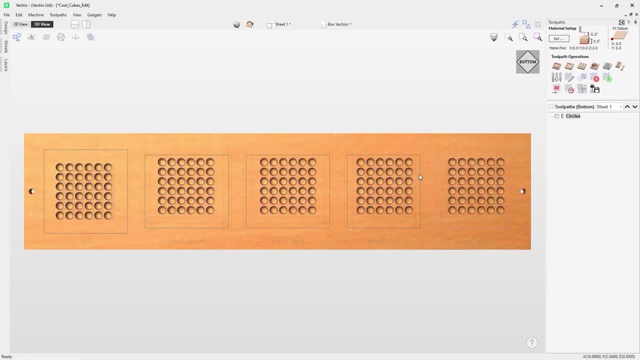 then we'll go ahead and choose these last vectors that we need. holding down our shift key. we can select all of those outside profile boxes, create a profile cut. in this case, our startup is going to be at zero. we're going to cut all the way through our material. so I can. 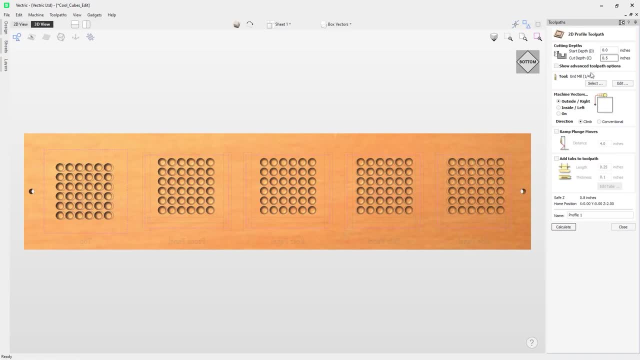 just type in Z and press equals on my keyboard. we'll use that same end Mill. we're going to cut outside those lines. we're going to add in some tabs. if we have a look at our 2D view second, you'll see that we have tabs in our 2D view and these came from the original. 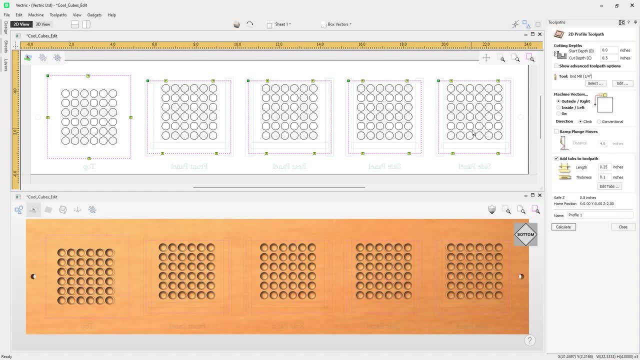 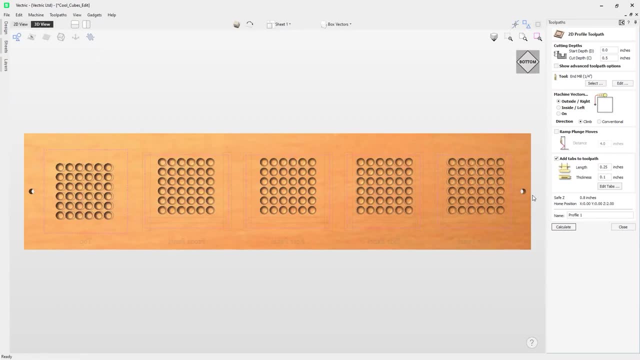 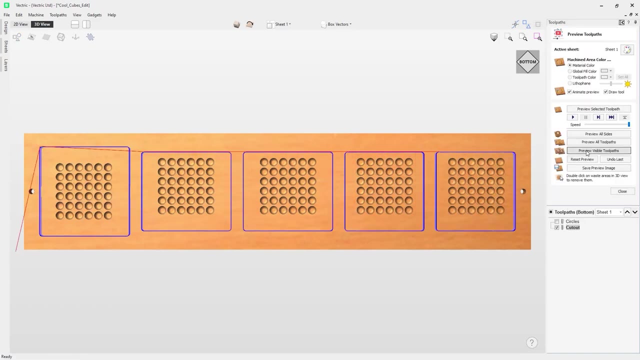 file that was created and I'm pretty happy with those. If I want to go ahead and adjust those, I can. I think those are great just where they are. Let's go ahead and maximize our 3D view again. We'll call this Cutout and we'll calculate that. We'll preview our 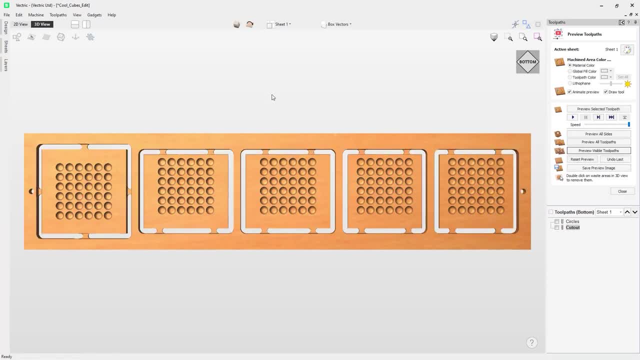 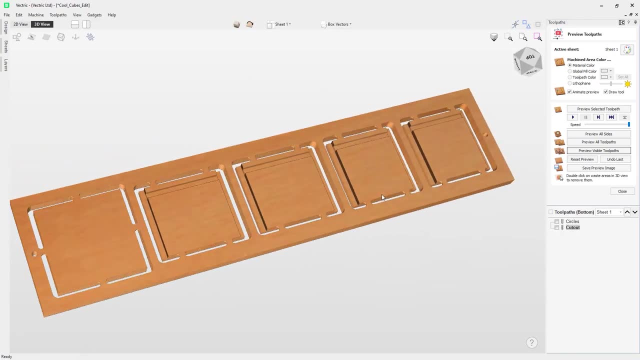 visible toolpath and because we have our double-sided view turned on as we go ahead and rotate this around, we'll see that we can see both sides of our project at one time, making sure that everything lines up and at this point, if I'm not happy with the results, 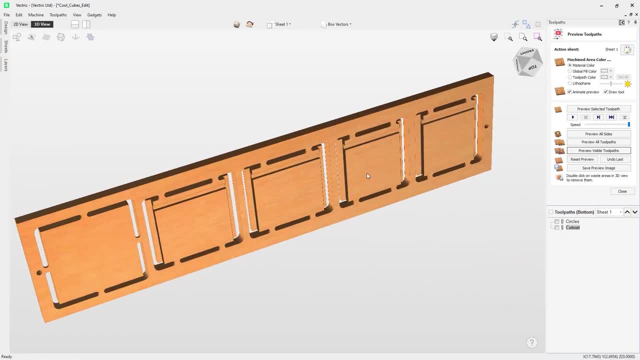 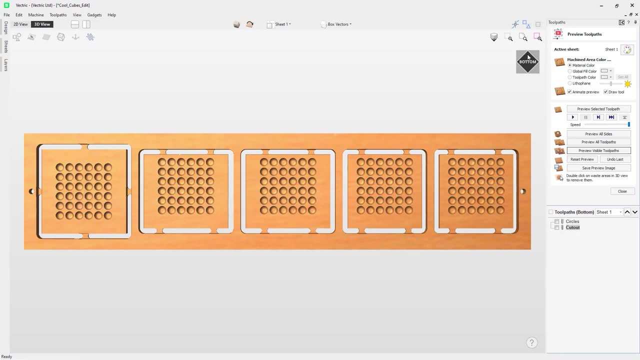 I can go ahead and reset up my toolpaths, change my vectors or do whatever else. I need to make everything look correct before I go ahead and save these off and run them on my machine Now. one more thing I want to show you about a double-sided job or a two-sided 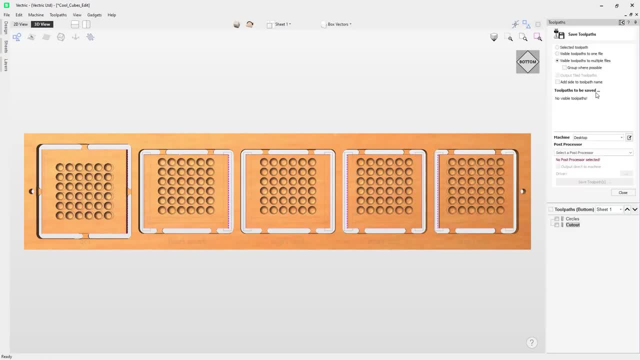 project is that when you go ahead and save off your toolpaths you have a new option that says Add side to the toolpath name. So if we turn on all of our toolpaths, we make sure that that is turned on. If we go ahead and choose a post processor for our desktop machine,